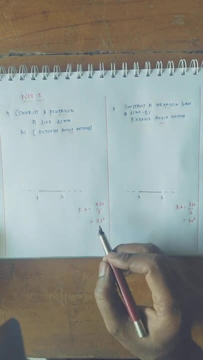 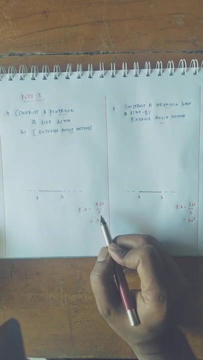 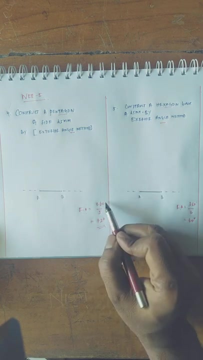 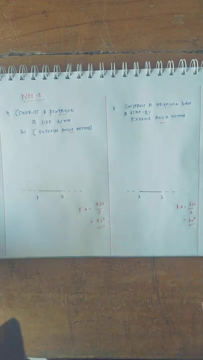 So here the simple concept to draw an exterior angle. it's nothing but EA is exterior angle. it's completely 360 degree. for a pentagon: 5 numbers of sides, 360 divided by 5, it may be 75.. Similarly, external angle for a hexagon: 360 divided by 6, total numbers of sides is 6, and this is 60 degree as considered as a external angle. 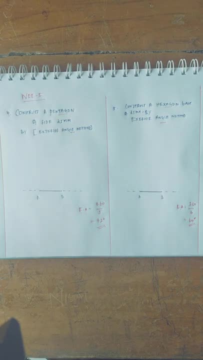 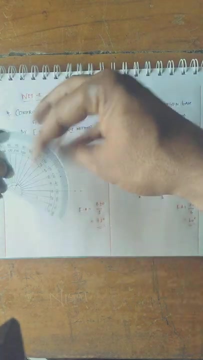 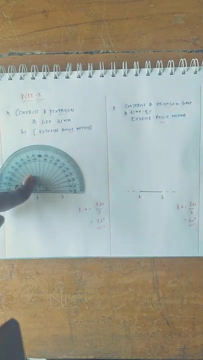 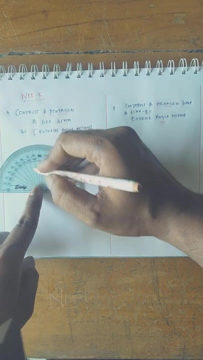 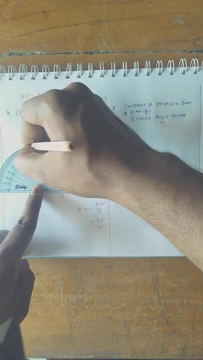 So initially I am dropping 2 numbers of sides. So let me draw a line as consider as a base that could be. that could be base of the pentagon and hexagon. So let me make a angular line that's supposed to be 72 degree for a pentagon. 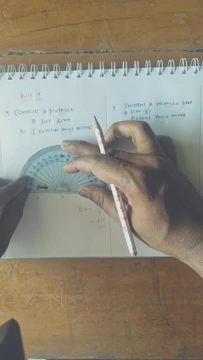 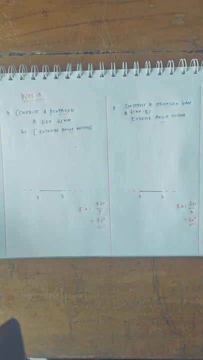 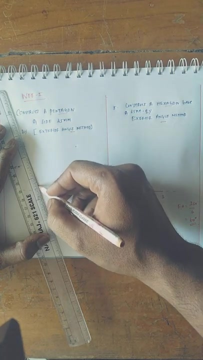 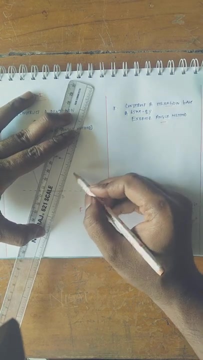 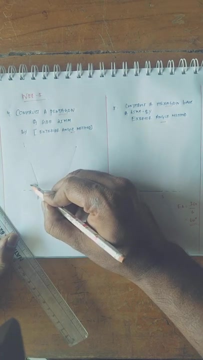 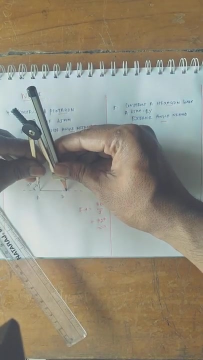 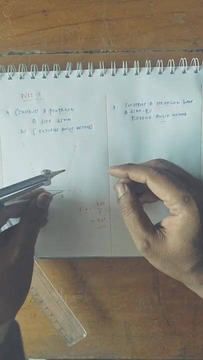 Similarly This side. it must be 72 degree. so let me make an inclined line considering outer. so these two sides, I am making 72 degree angular line from here, only With respect to horizontal, that is 72 degree similarly other side. So I am measuring the base 25 mm for a pentagon. I am intersecting this both angular line. I am keeping that same edges A and B. 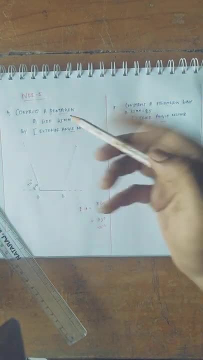 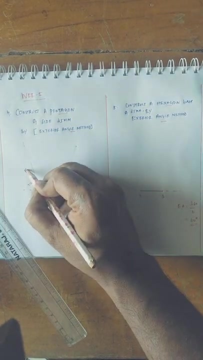 So now we need to identify the third point for the pentagon. let it be C. here there may be E, see D. here may be E, Io. and let me measure how. I just seems we need to find that another point, that is E. Sorry, do we measure this? 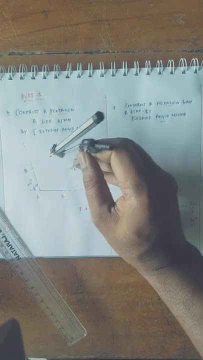 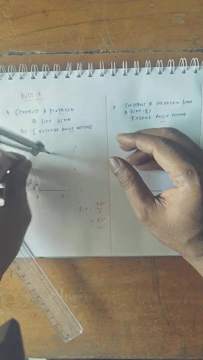 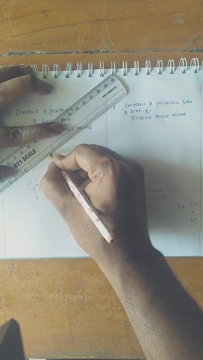 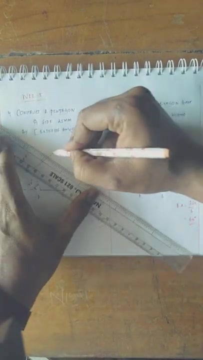 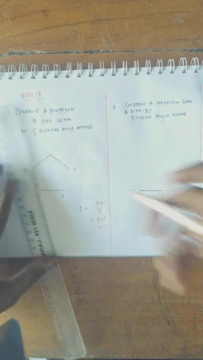 be Here. The same dimension. I am making ansar with CSS center. Similarly, I'm just making a NAR II. as a senator, You connect these two. that will use you the sites of the Sites of the Pentagon Sites. you need to connect, otherwise you may not get 25 mm length. So this is a complete pentagon. 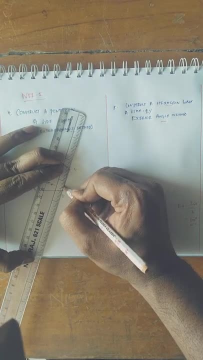 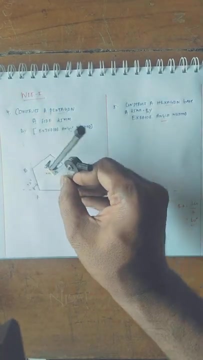 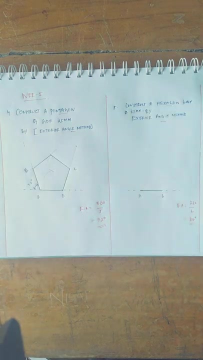 you need to draw. ok, So center for the pentagon. to identify the center for the pentagon, simply keep B as a center, A as a radius, simply mark here, and A as a center, simply make an arc, So that point could be the center, geometrical center for the pentagon In another way also. 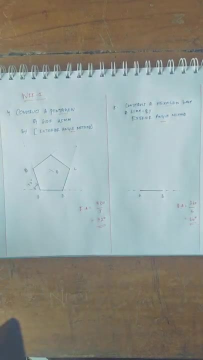 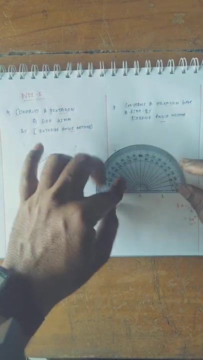 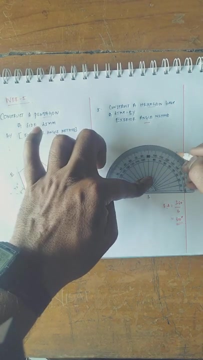 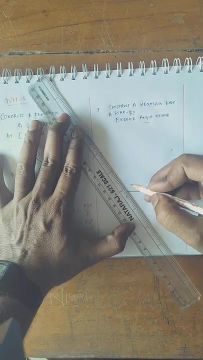 you could able to identify the center. Similarly, the exterior angle for an s. second, we need to take 60 degree, 60 degree and similarly, at B is 60 degree. fine, Now we just connect these two lines. you not to connect much, just make a line for a certain. 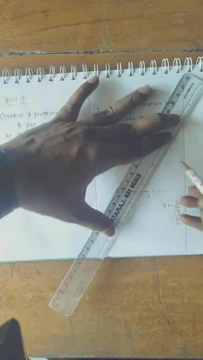 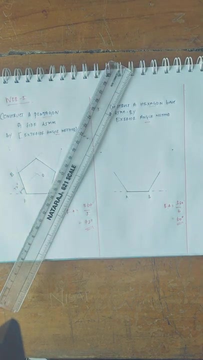 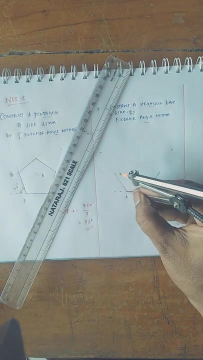 distances, it is sufficient. otherwise it is over righted and raising itself still. it is complicated. now you measure A, B is 25 mm and keep A as a center, 25 mm as a radius. similarly B as a center, 25 mm, 3.33 mm As a radius, 25 mm As a radius, 1.25 mm As a small belt like this, while the & puff. 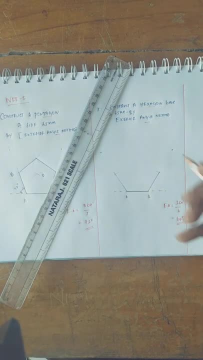 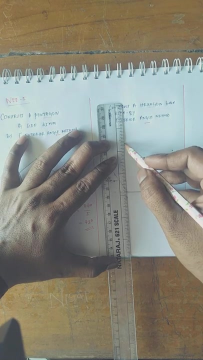 Now we got two points that you can name: A, B, C, D will come here, E will come here F. I am specifying these two points are F, So remaining two points we need to identify, for that you are at a vertical line from A and you are at a vertical line from B. These 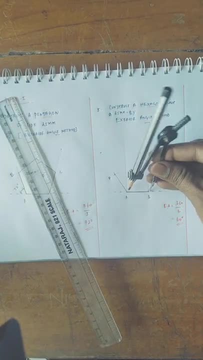 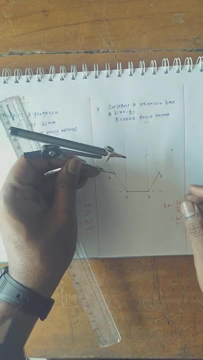 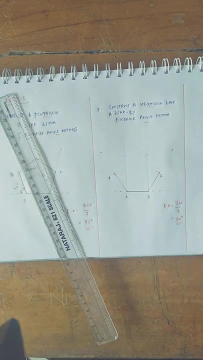 two should be parallel. Now again, the measured angle: 25 mm- and keep C as a center and that vertical line as a radius. 25 mm as a radius, you intersect that vertical line. Similarly, keep F as a center and intersect that vertical line. So this is D, this is E. So if you 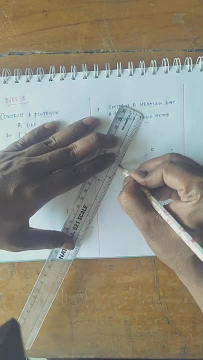 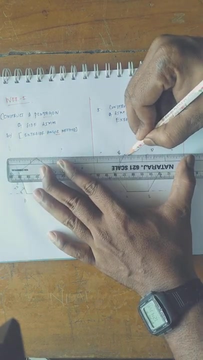 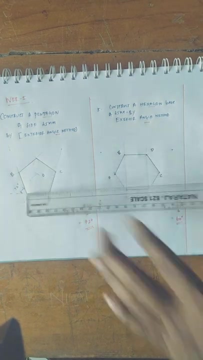 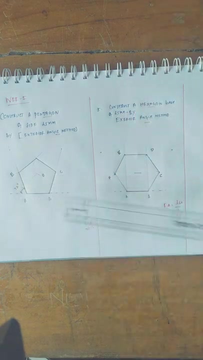 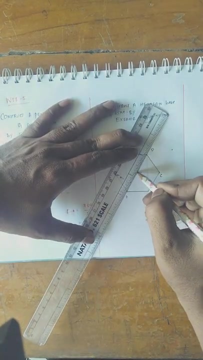 are connecting it. So Now you may get the regular hexagon. that is it quietly simple. So to identify the center for the hexagon, it may be otherwise. if you are making a diagonal this point, we are making a diagonal.